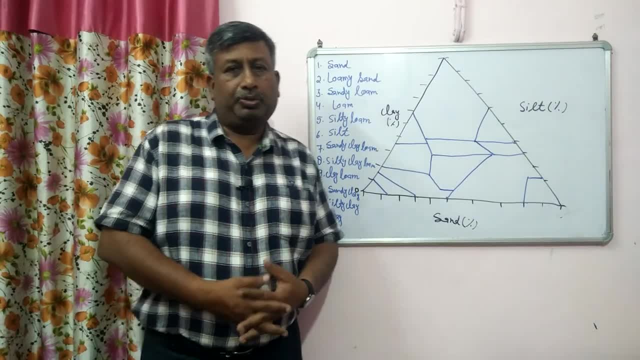 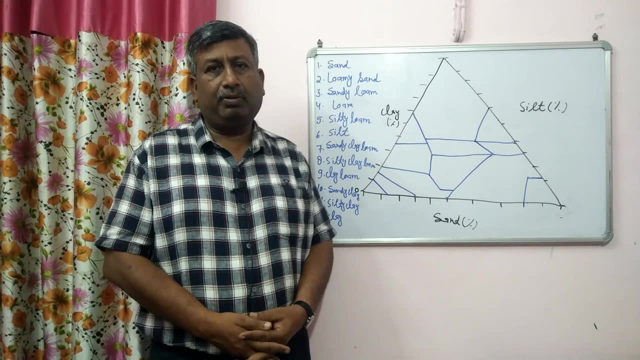 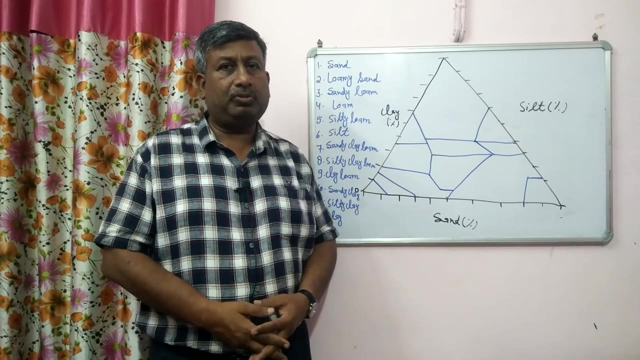 Hello students. I am Dr Amit Bhatnagar, professor in the department of agronomy at GB Pant University of Agriculture and Technology, Pannagar, Uttarakhand. What is structural triangle and how to determine the soil texture? The soil texture is very important because it affects the soil physical. 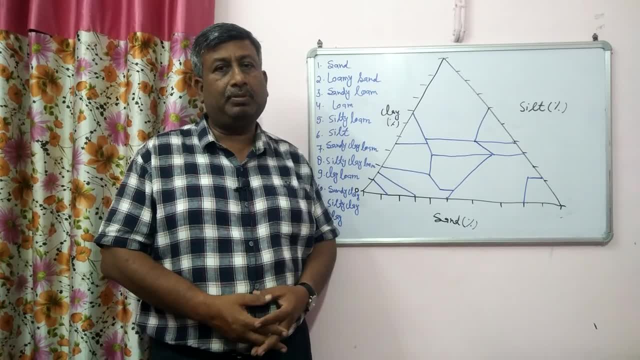 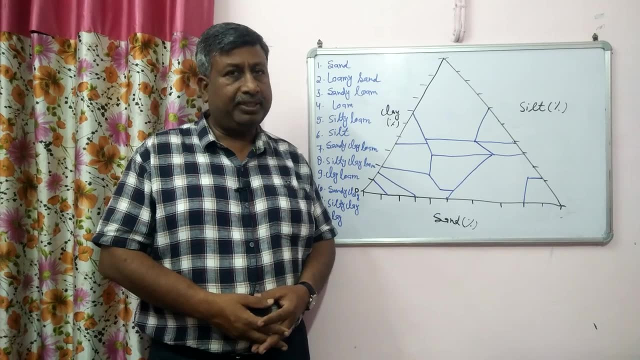 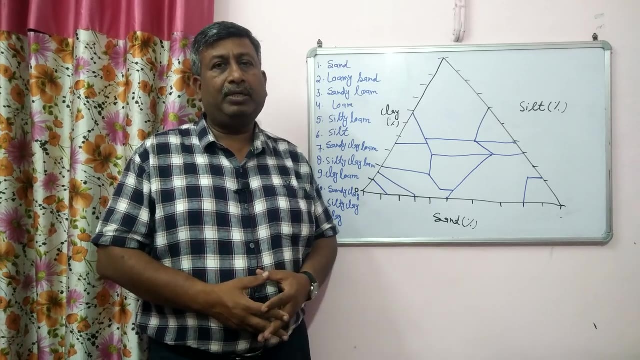 properties and soil texture is relative proportion of sand, silt and clay means what is the percentage of sand, silt and clay? it decides the soil texture and a triangle is used to determine this soil texture. First of all, we have to find out what is the percentage of sand silt. 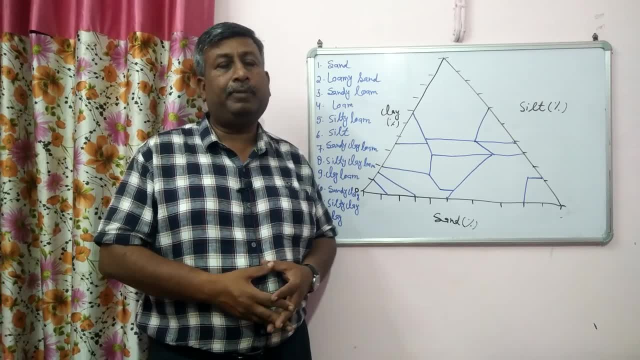 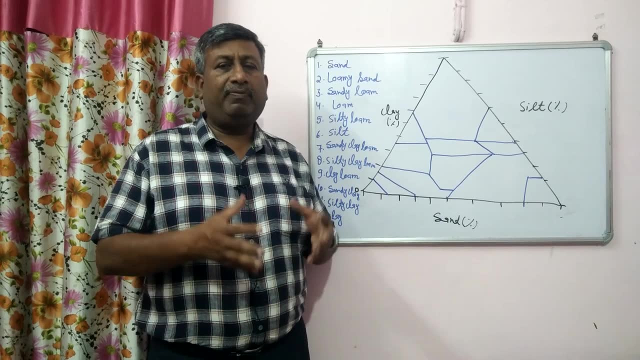 and clay in soil. So first of all we have to find out how much is sand, silt and clay, and for this we do mechanical analysis, and when it has determined that this is the percentage of sand, silt and clay, Then this triangle is used. 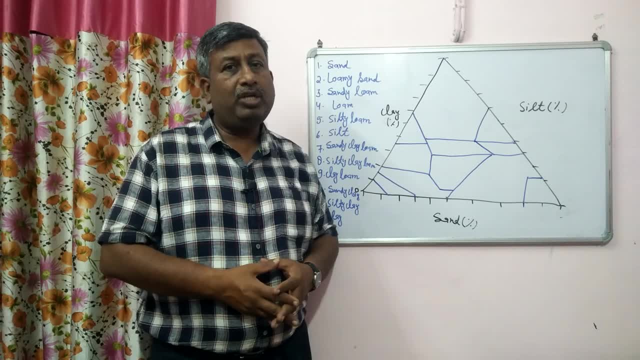 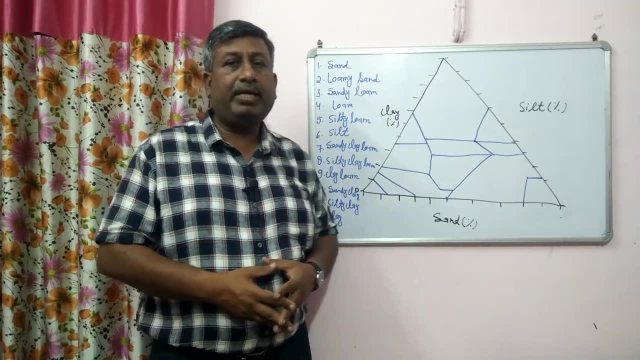 So these are the first four elements to determine the soil texture and there are 12 soil textures. I have written all the 12 soil textures and this is the Triangle and how this triangle is used and how the question may be asked from this triangle. I will explain. 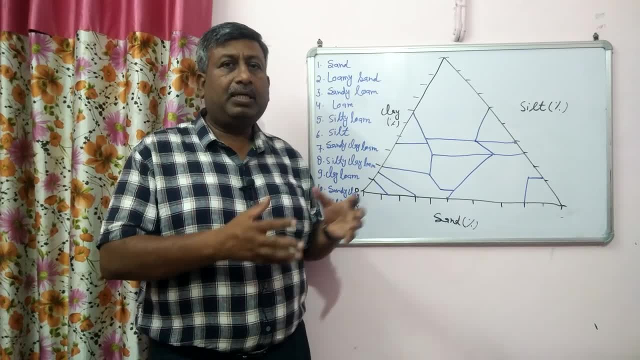 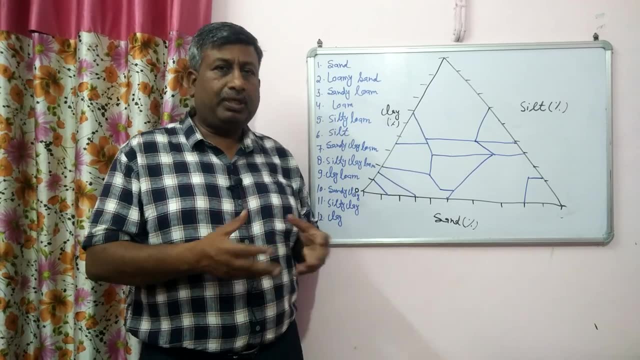 So what is a texture triangle and how to use this? First we get to know about the soil of our field. what is the soil texture? it is fine, coarse medium. physical properties are regulated from it And in examinations also we get to. 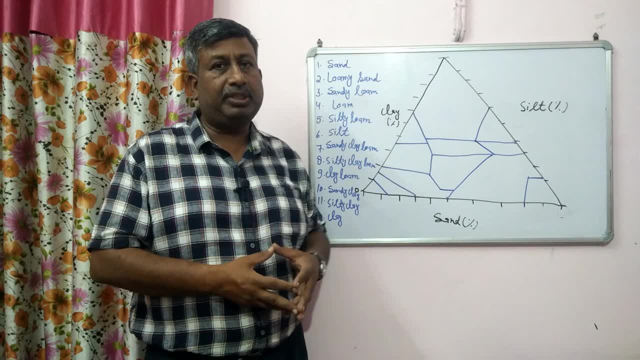 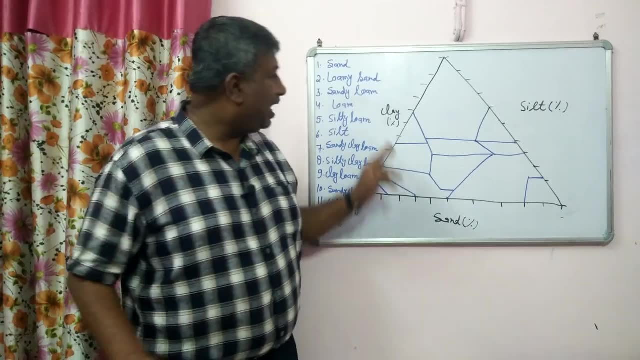 question: puche ja sakte hai ish structural triangle se ki ish ko kaisi use karte hai? toh this is equilateral triangle, means all the three sides are equal and on the left side clay is written, clay percentage, on the left side and the right side silt, and at the 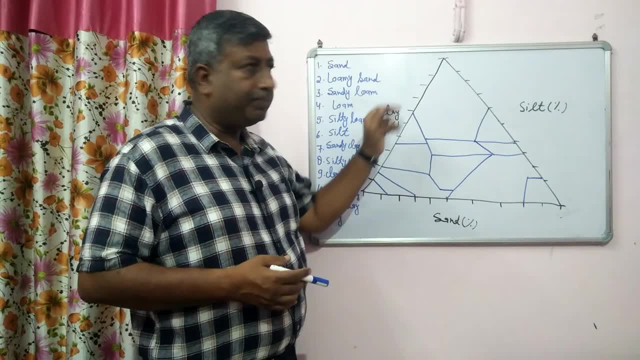 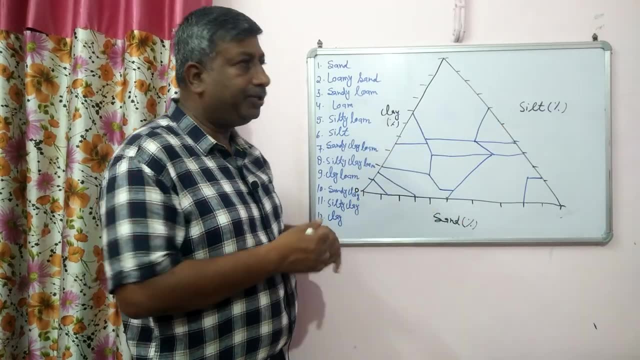 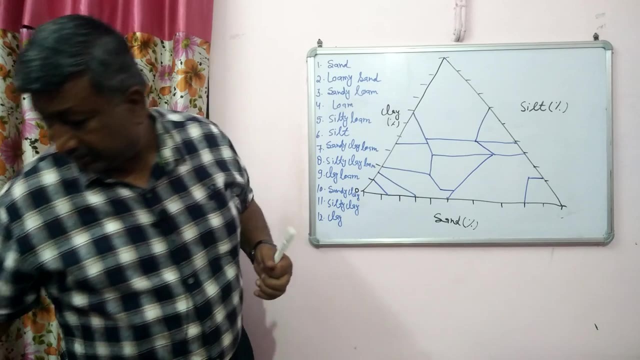 base sand tom pehle ek equilateral matlab sum bahut rujek banate hai. uske left side me hum clay percentage ko denote karte hai, right side me silt ko aur jo base usme sand ko. then each line is divided equally in ten parts, and this is started, this clay is started. 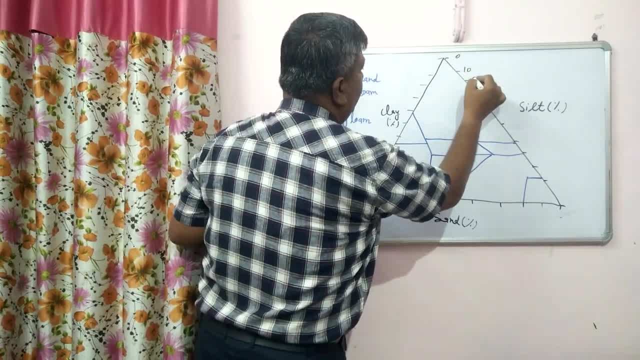 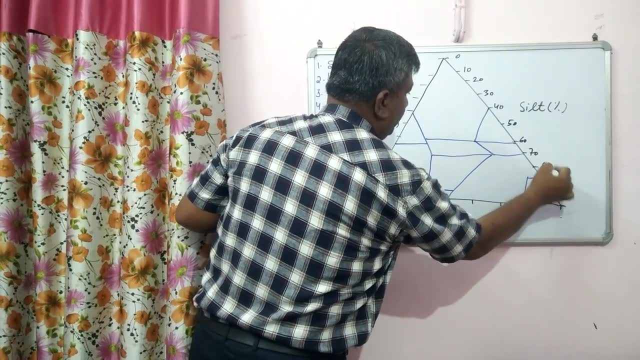 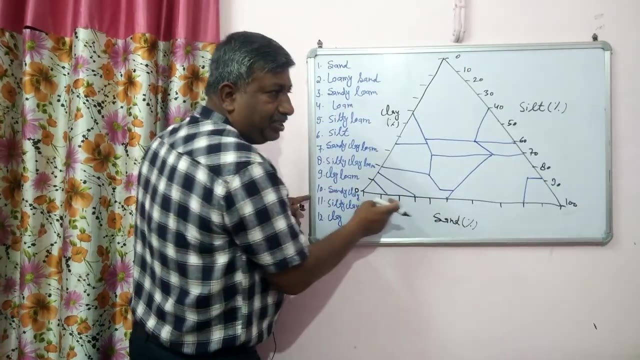 with the here at zero percent, ten percent, twenty, thirty, forty, fifty, sixty, seventy, eighty, ninety and hundred, and then sand is start from this side to this side. first is silt, then sand will start from this side. it means it is zero, then ten, then twenty, then twenty. 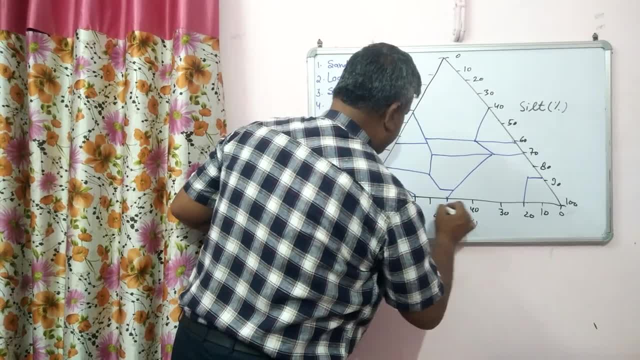 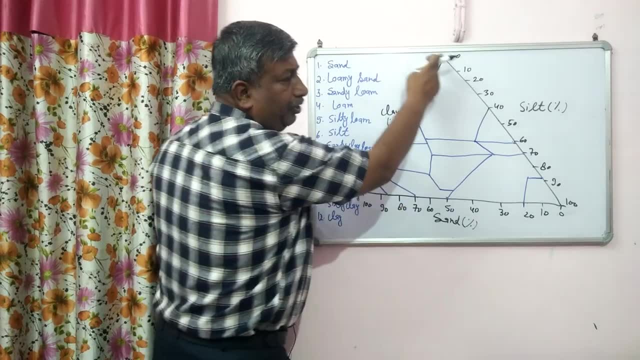 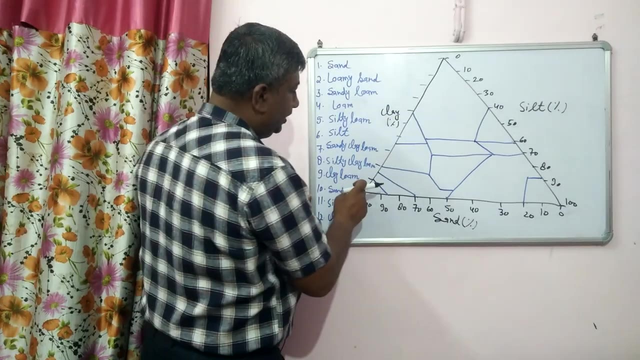 thirty, forty, fifty, sixty, seventy, eighty, ninety and hundred toh silt ko upar se start karenge and then sand theing1 nahan se meech safe. eh bottom se top pehchalenge clay ke percentage. toh yeah jo hai zero percent clay hai. this is ten percent. 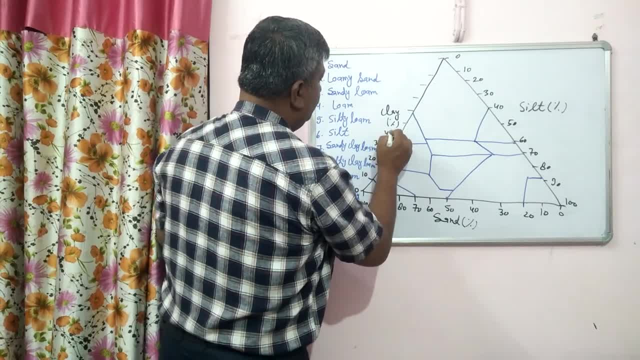 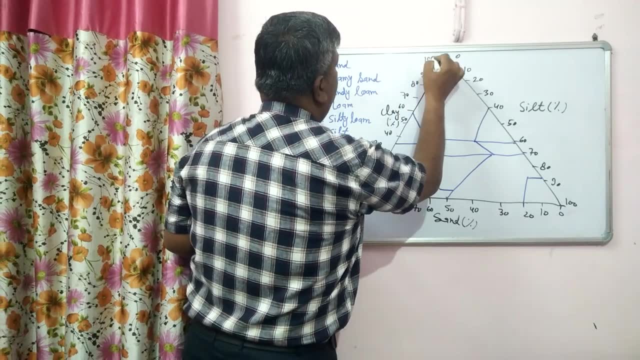 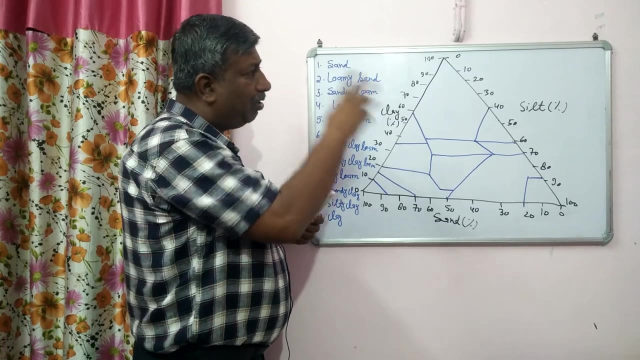 this is twenty, this is thirty, this is forty, this is fifty, this is sixty, seventy, eighty hundred 90 and this is the hundred percent. the first question to hecky: what is the type of the triangle? triangle is equilateral. triangle means all the three sides are. 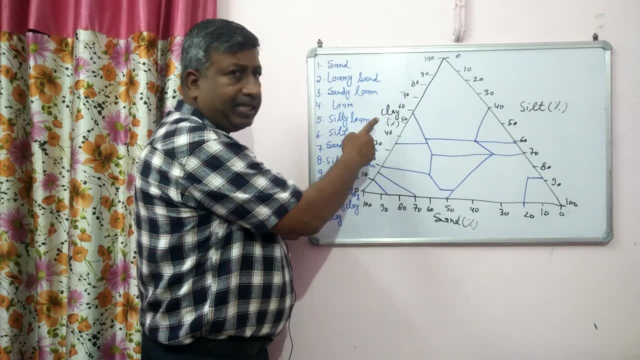 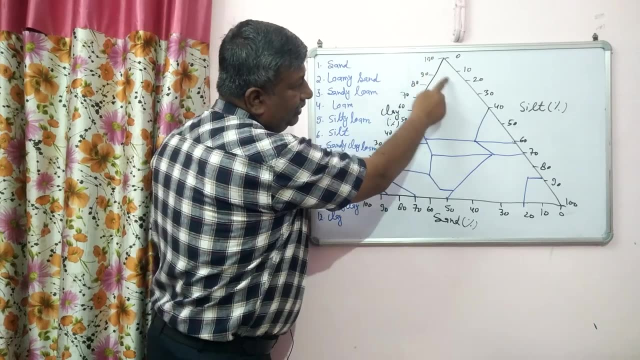 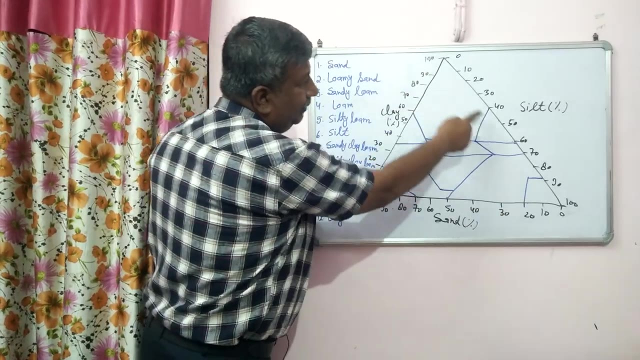 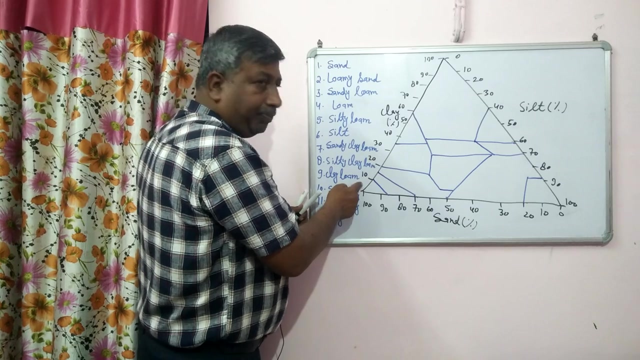 equal and where sand and silt is written on left side clay, then right side silt and on the base of sand and how the percentage return from top to bottom. it is increasing. top to bottom it is increasing. then right to left sand is increasing. and if we move from right hand to left hand then sand is increasing. and if we move from bottom to 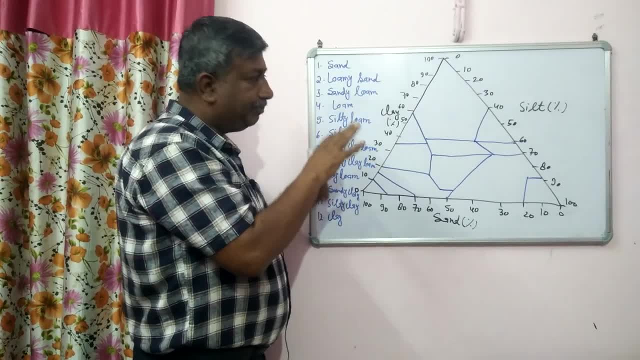 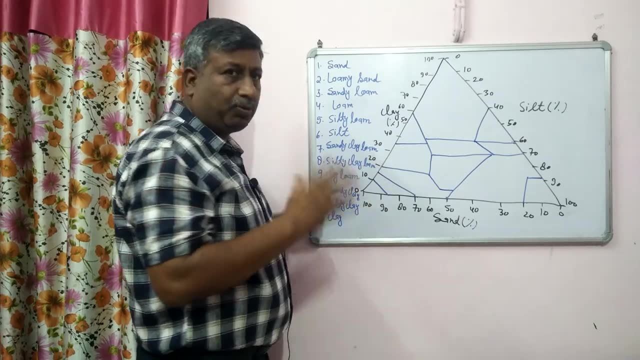 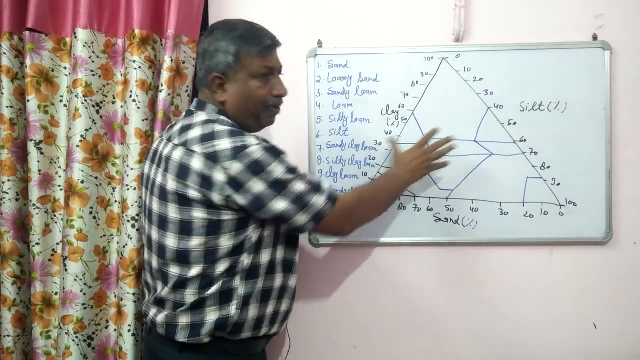 top, then clay is increasing. so this you should know in this way and this diagram is a little typical. this is a typical diagram. this will be given in book or in question paper. it is given in books and in question paper. also, no need to draw this type of diagram. this diagram will be like this, but 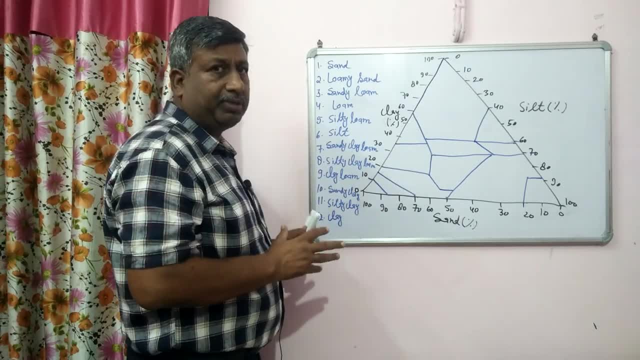 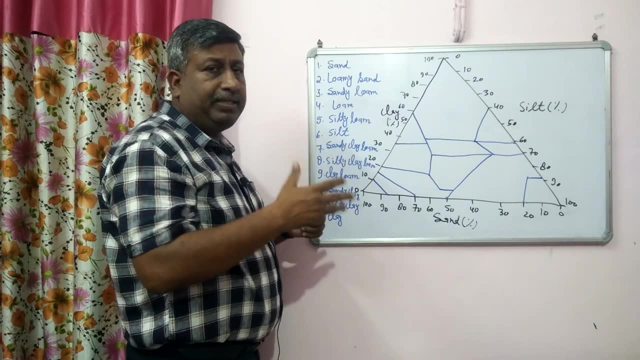 you have to number this diagram, how we do it. it very easy, meaning i do tell the numbering of this, how to do it and how this is written, which is how i will explain to you how to do it very simply. if you will see this lecture, then you can easily mark them: soil. 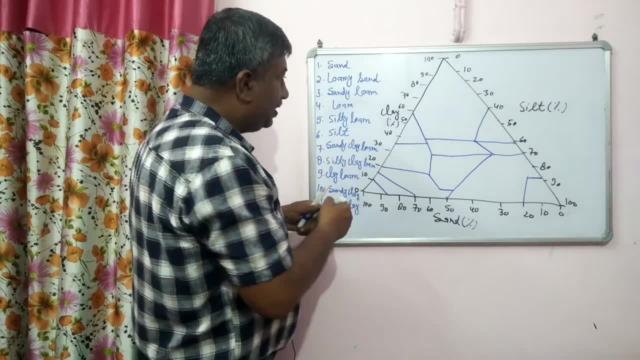 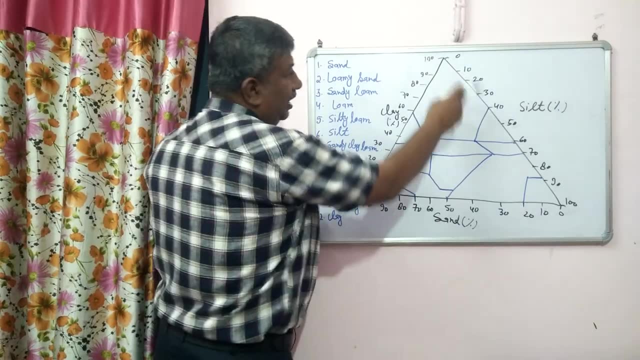 texture number and the soil class. so first start with the number, that is, start with a here. this gave the smallest part, so it give one number. this is the largest part to give 12 numbers because there are 1,2,12 textural classes. how many classes are there them? 12 textural class. so the 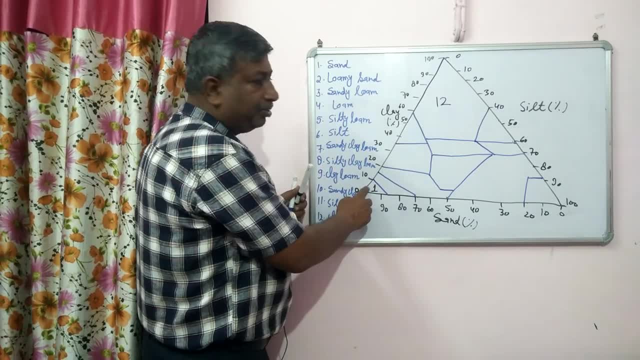 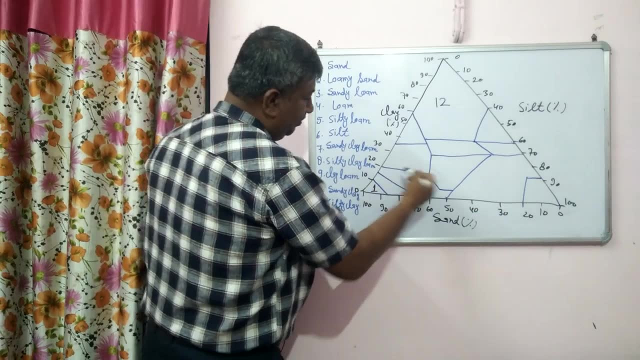 from 1 to 12 are the textual classes. so we have started from here. which is the smallest and the biggest, we have given 12, then start. we will start the numbering from here. we will start the numbering from this side: 1,, 2,, 3, 4. 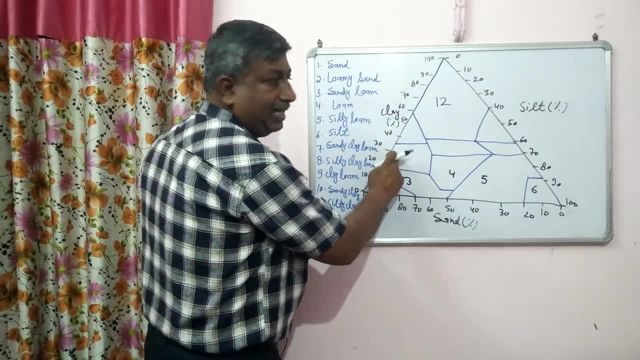 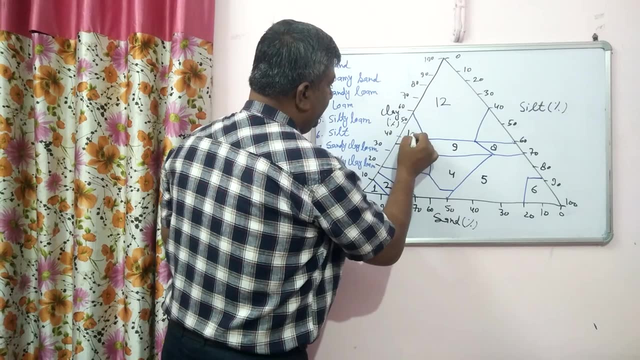 5, 6, 6 is completed. now we will come from here 7,. why do we have to do this? we have to jump 8 and 9, then 10, 8,, 9,, 7, 8,, 9, then 10. 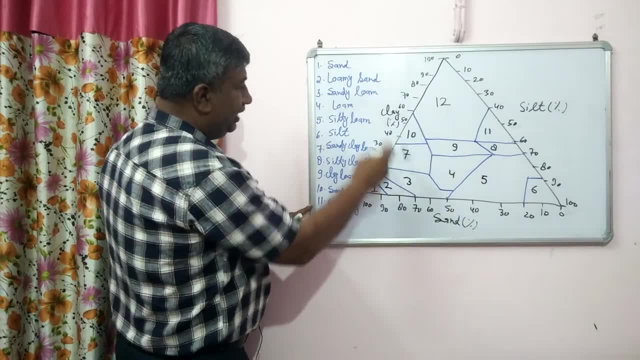 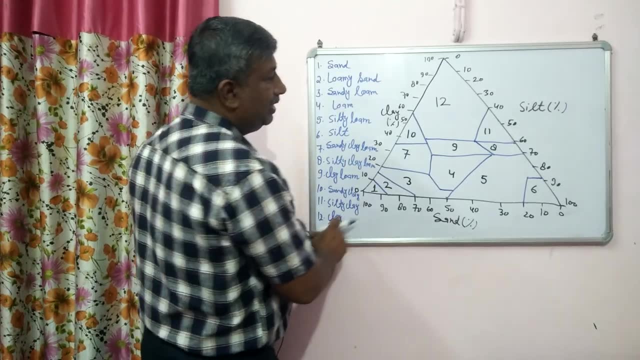 then it is: rest is 11. now, 1 is sand, 2 is loamy sand, 3 is sandy loam. likewise, 9 is clay loam. 12 number is clay soil, 6 number is silt. so this is the numbering and the 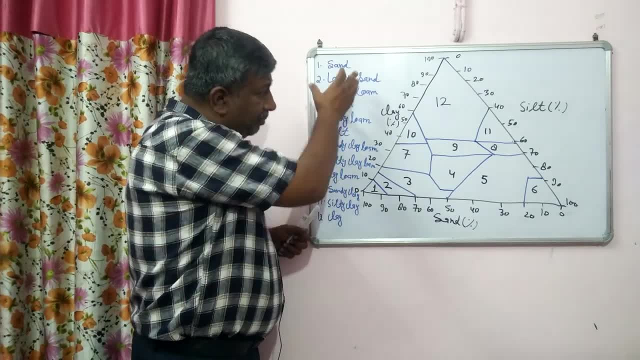 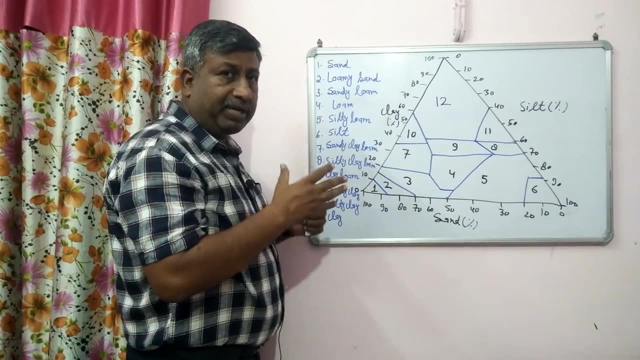 textual classes and how this textual classes are written. I will tell you how it is written, how we determine it. so this is the textual triangle which is very, very helpful in determining the soil texture: 1,, 2,, 3,, 4,, 5,, 6,, 7. 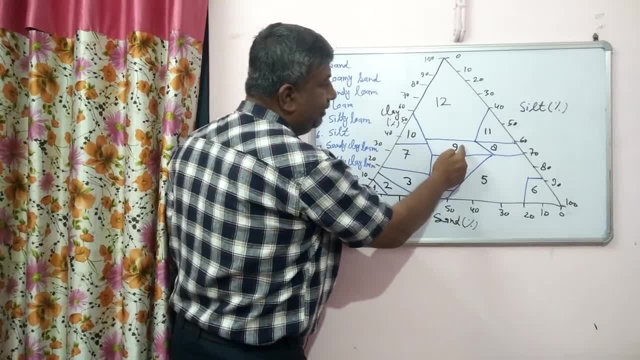 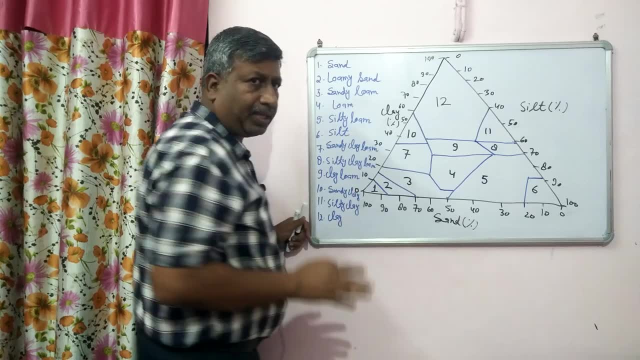 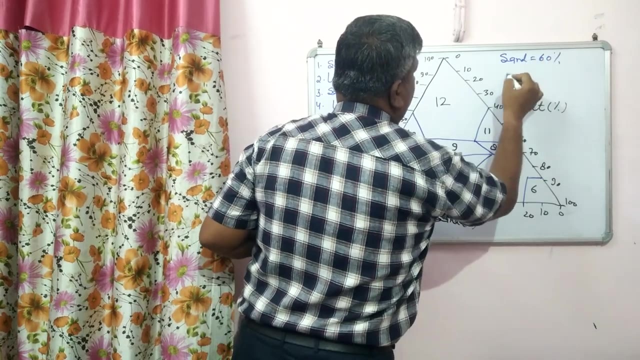 what you have to do here. you have to scoop 8 and 9, then 10, here is 12, so the rest is 11, and this number will come in this textual class. now, suppose this soil, this soil has sand. suppose sand 60% and 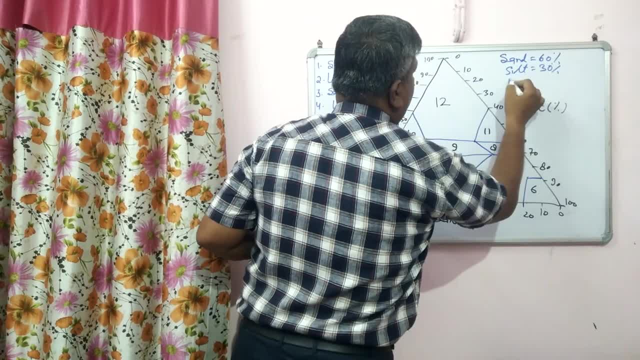 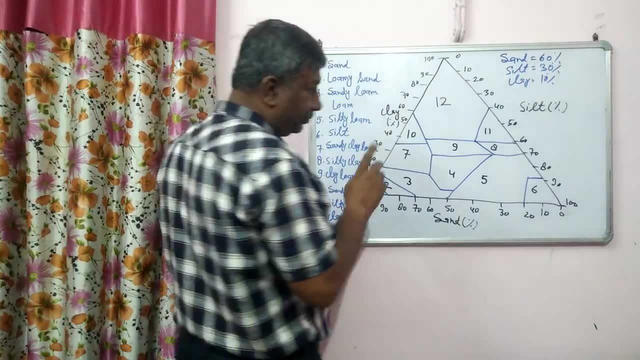 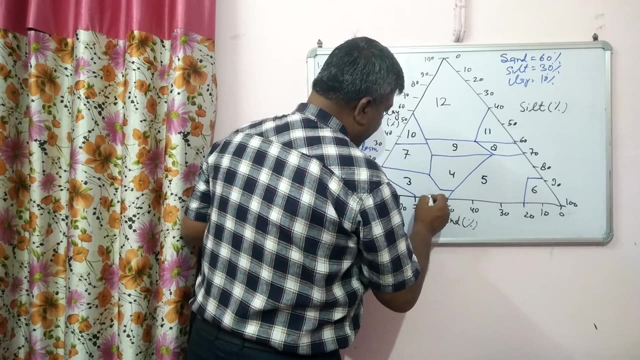 silt, suppose 30%, and then clay, automatically it is by 10%. so what is the texture? what is the texture? first, this is the sand. so sand has come on 60, then mark the 60, 60 and then the sand is moved diagonally upward in this. 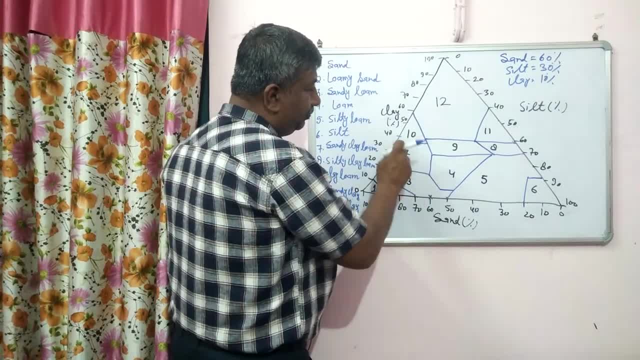 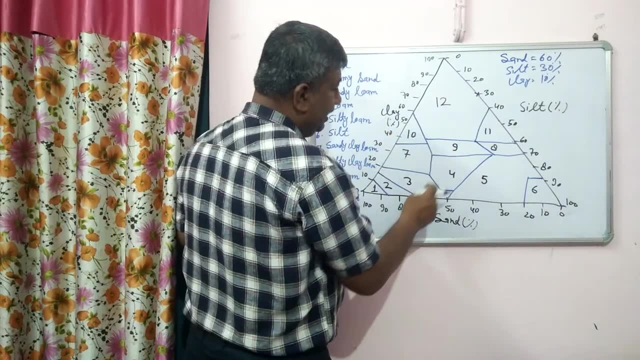 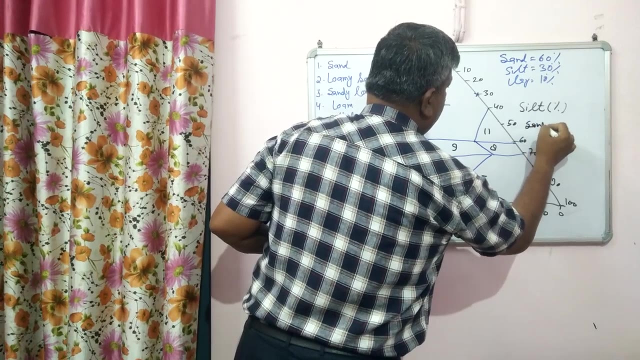 way. we will move sand, we will mark it on 60 and silt is 30%, we will move it on 30, so we will move sand parallel to silt. now you see, it is written as sand, silt clay, it is written as sand. 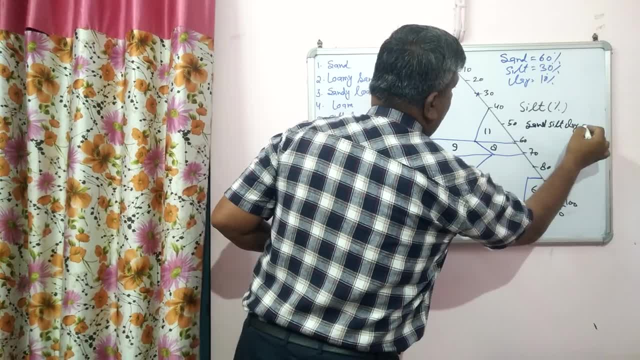 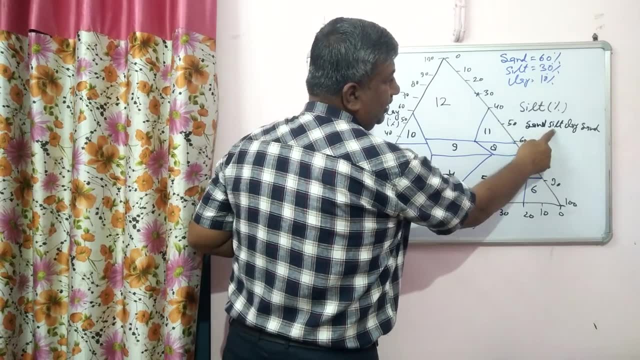 silt clay, again sand. so this is the generally we call it sand, silt clay. so if we will move on sand we will move on silt. silt will move on parallel to clay. if in clay then it is parallel to sand, we have to move on sand. so where? 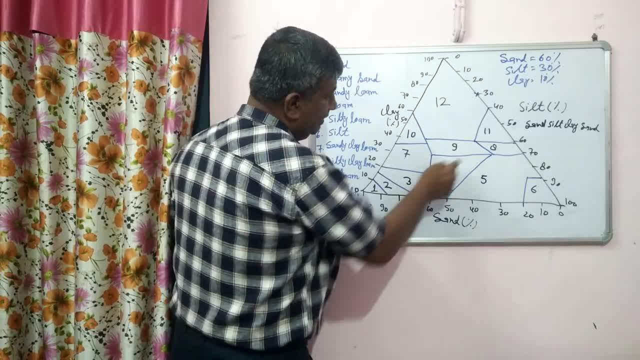 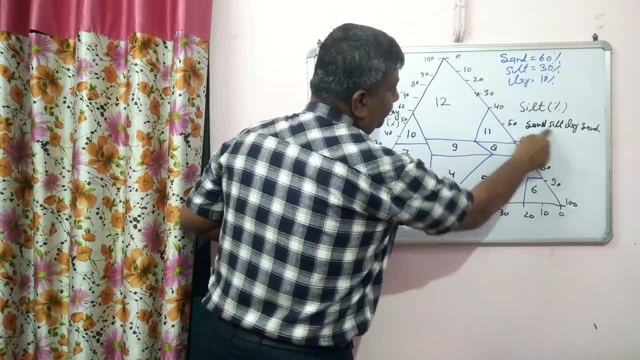 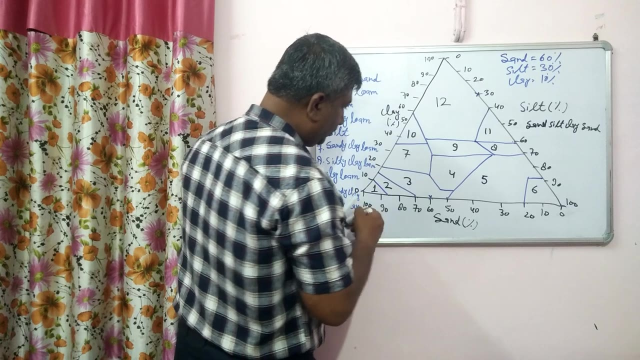 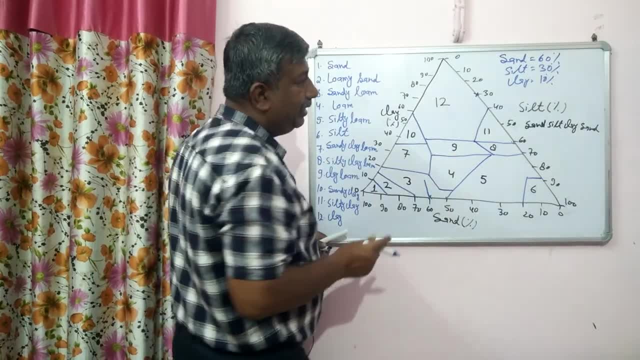 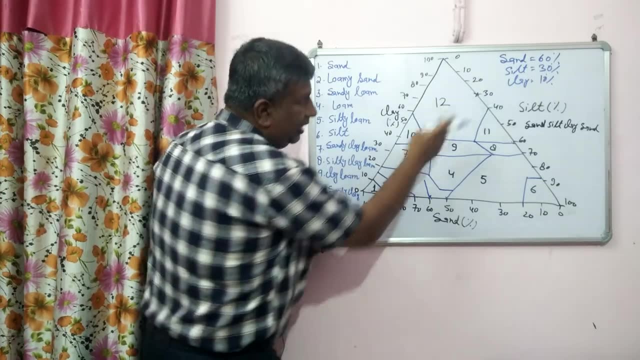 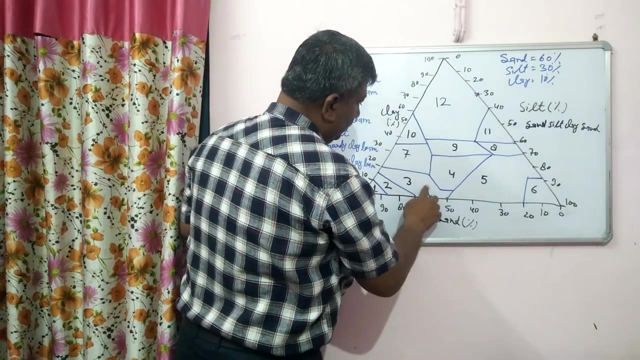 diagonally parallel to silt. ok, then it is the 30% silt. now, after silt, we will move parallel to clay. clay is like this, so we will move like this. we will not move like this parallel to clay now, we will move on parallel. 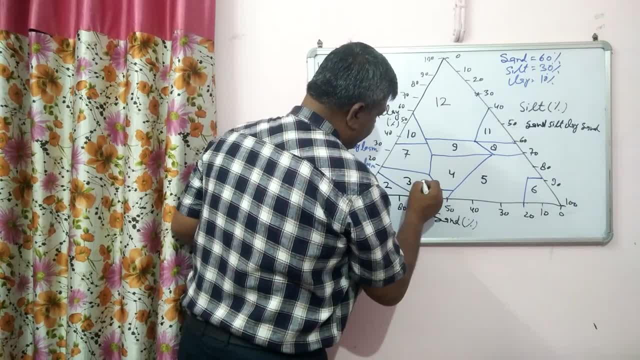 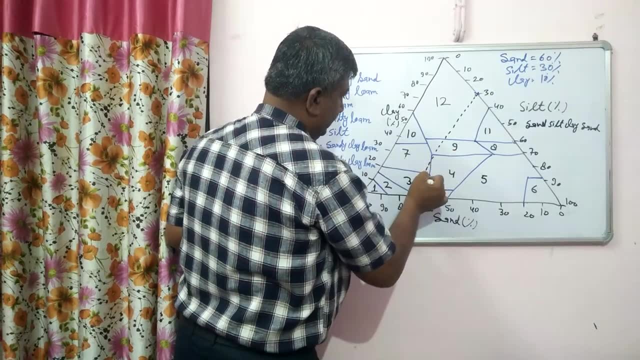 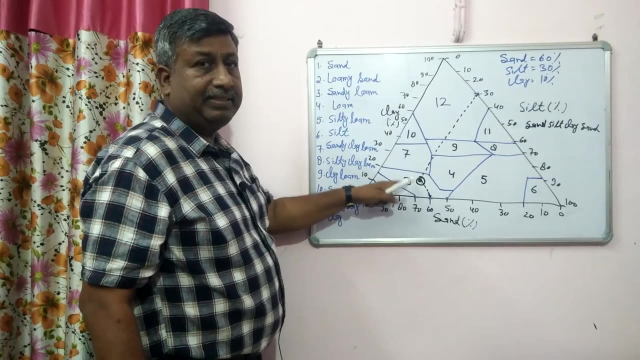 so I will show it with dotted line. it is: sand is parallel to silt and silt is parallel to- and this is this is the intersection point. so soil is in third group, and third is sandy loam. so soil is sandy loam. again, we have understood how to determine. 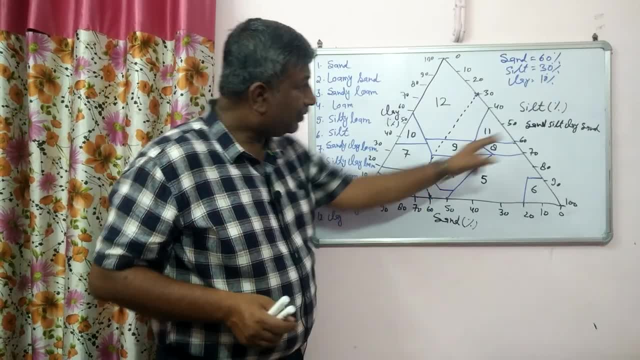 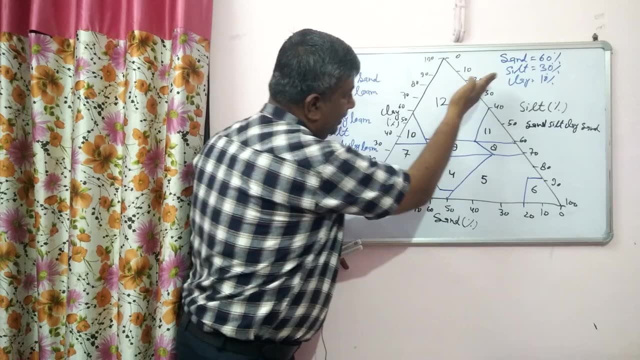 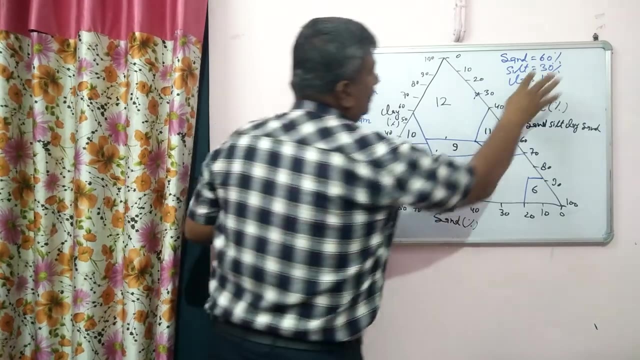 put the mark on sand, put the mark on clay, then move sand parallel to silt line. we have to move this and then silt move parallel to clay. another example: we will take another example: sand, silt, clay. we will change it and suppose it is 20%. 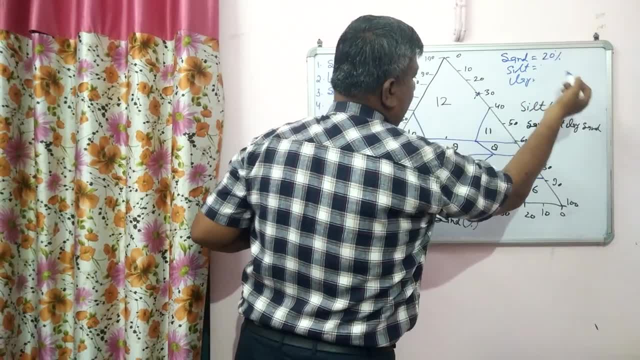 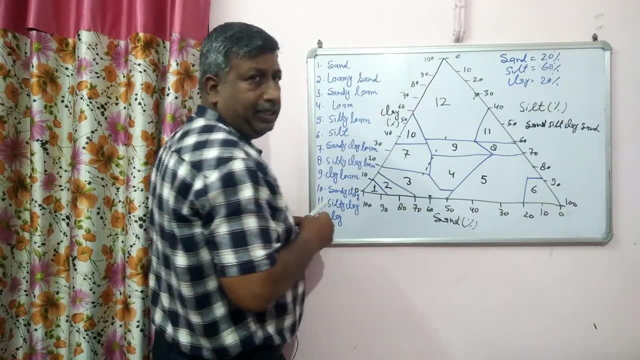 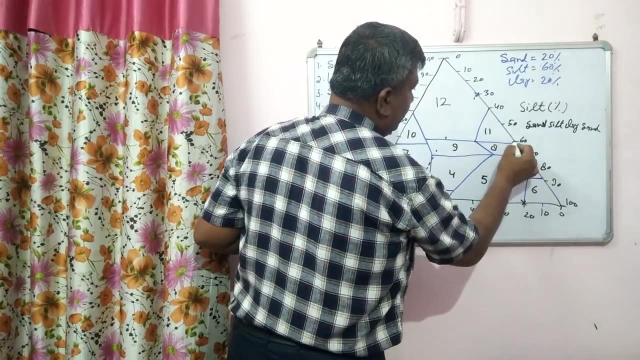 sand is 20% and silt is suppose 60% and remaining clay is 20%, then what is the texture of the soil? so sand, mark sand on 20%, then mark silt on 60%. now how we will move it? we have to move sand parallel to silt. 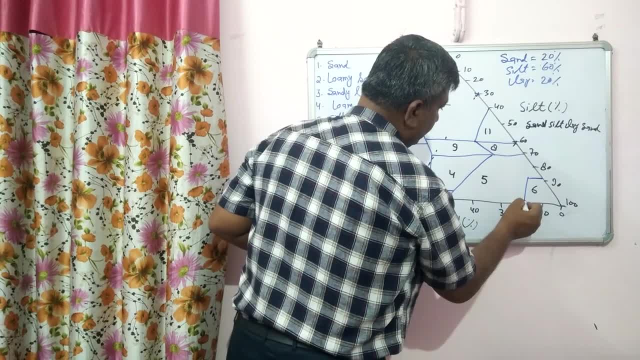 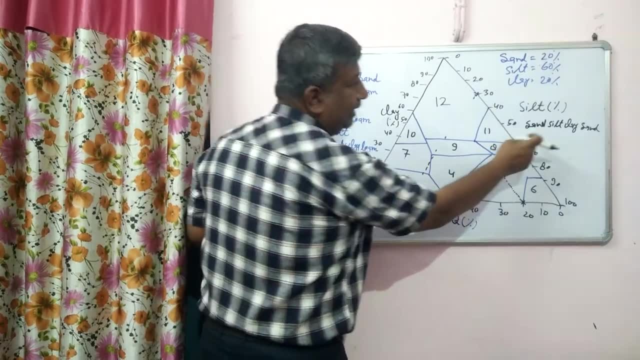 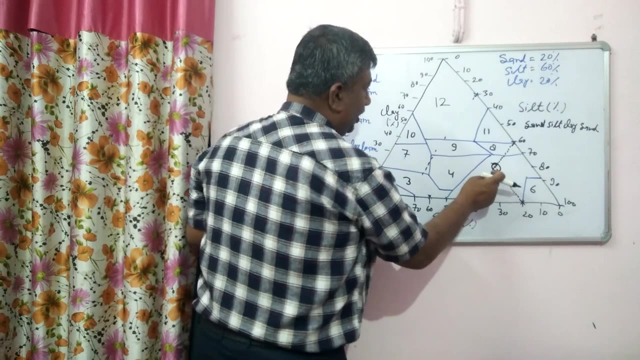 so this is silt line. we will move it like this. we will move it like this and then mark 60. now how we will move it on 60. we will move it parallel to clay. this is the intersection point. so this is the soil group. so this is in 5. 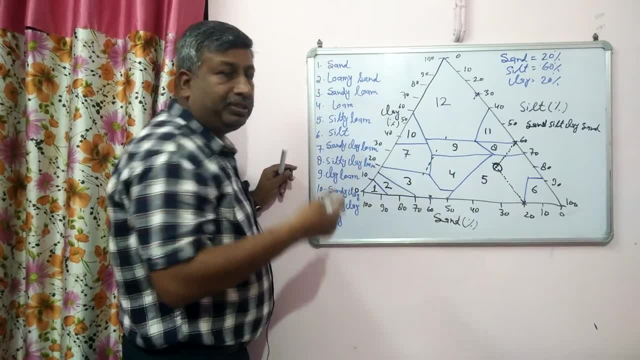 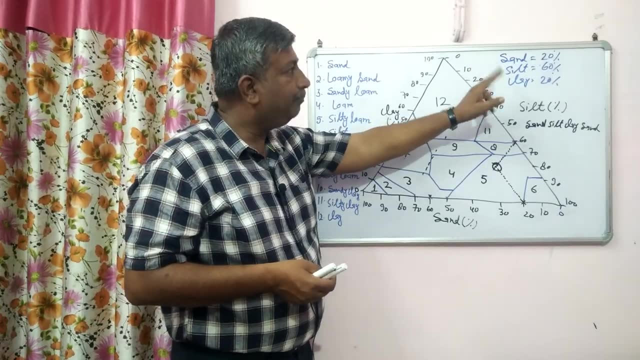 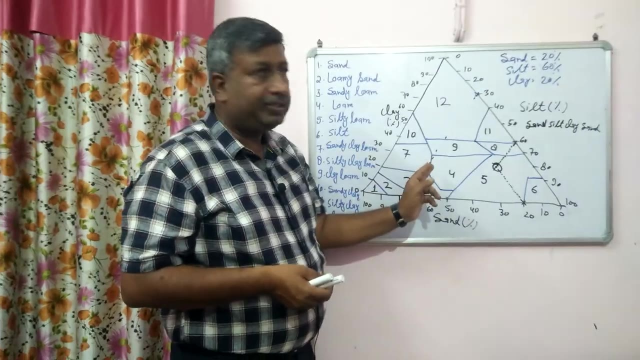 it is silt loam soil. so this is the way how we can determine different type of texture classes. we have to keep the proportion of silt clay. we will use only 2, because third will come from subtraction. mark on sand. mark on silt: sand line will move parallel to silt. 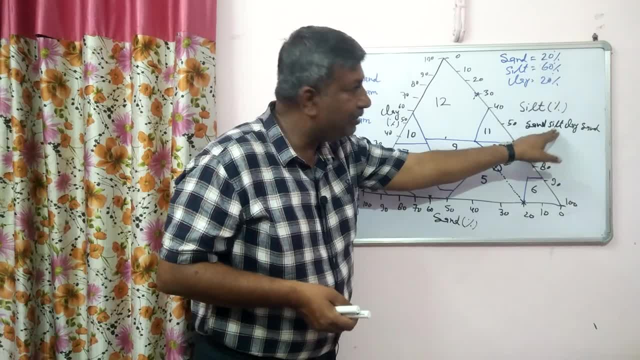 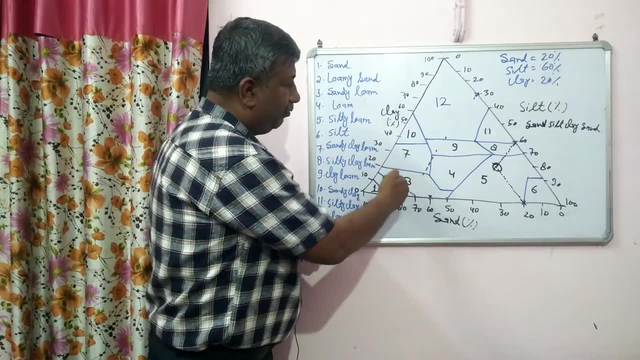 and silt line will move parallel to clay. see, i have written sand, silt, clay. sand sand will move parallel to silt and silt will move parallel to clay. so this is how we can determine texture class. so this is the way numbering 1,2,3,4,5,6,7. 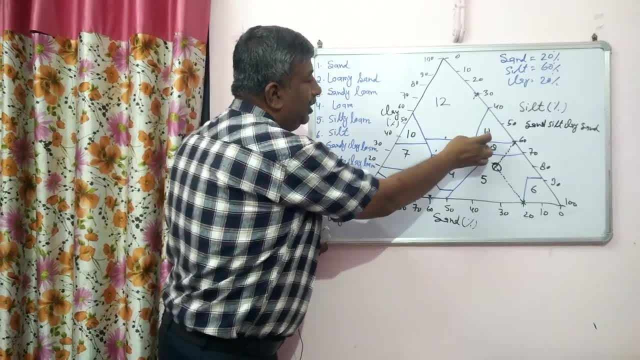 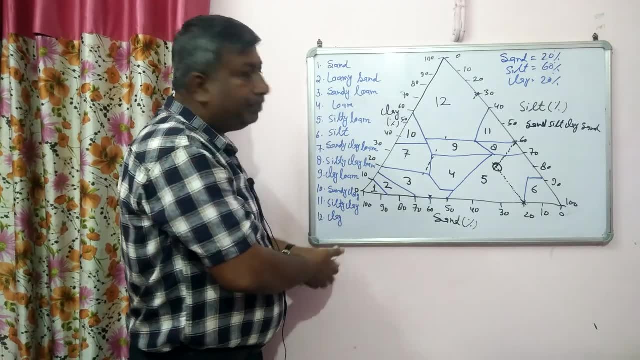 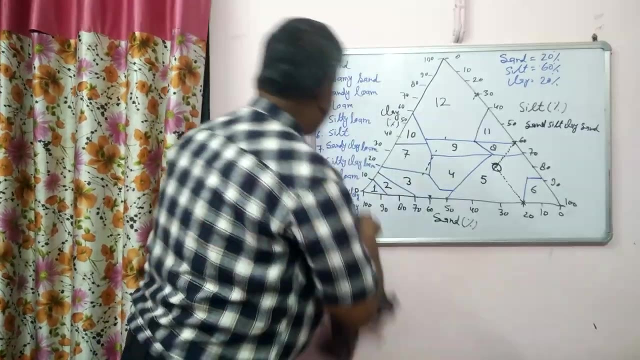 then jump 8, then move 9,10, then it is 11. now question is: how to give the name. how to give the name. so first you have understood textual triangle, how to use it. now how to give the name. there is a trick you will never forget. 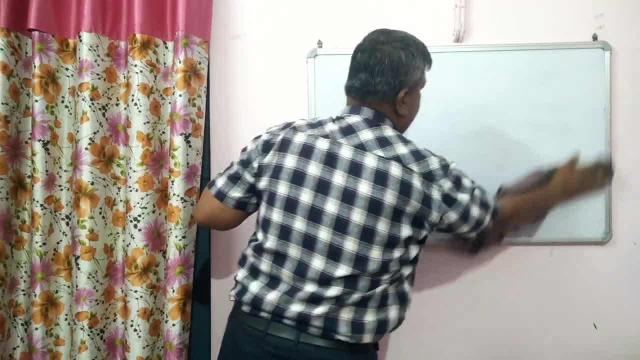 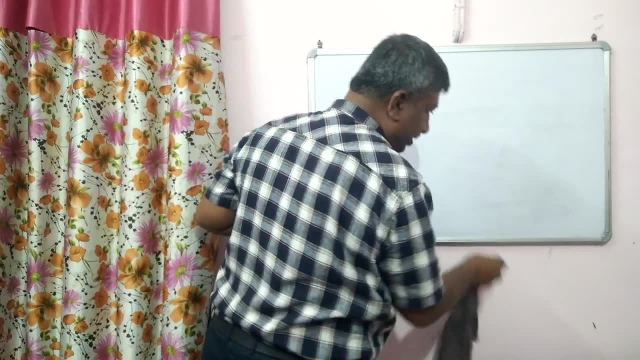 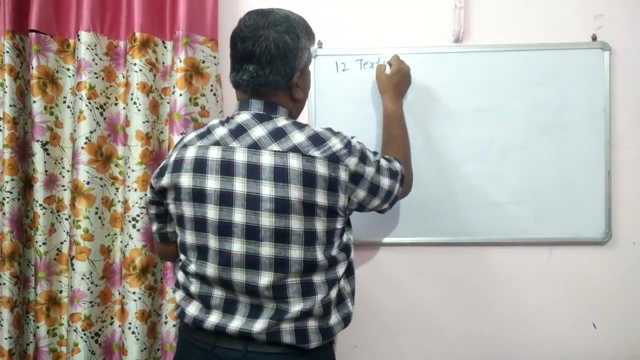 and this trick is easy, not tough, but you have to be careful. and this 12 textual classes from chorus to finest group, from the most coarse to the finest. there are 12 textual classes from chorus to finest. there are 12 textual classes from chorus to finest. 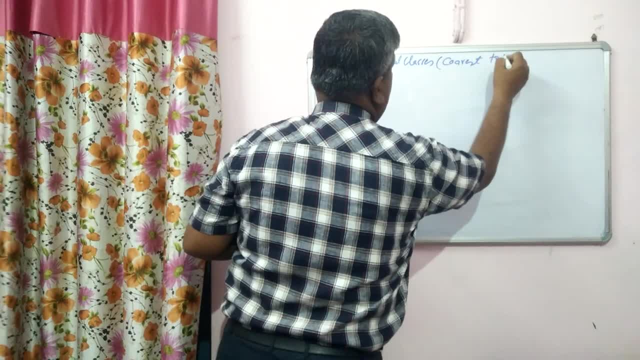 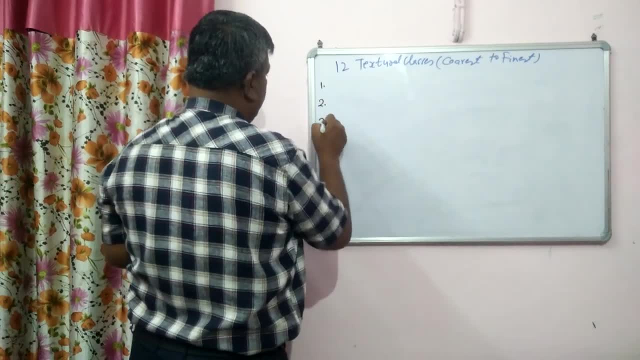 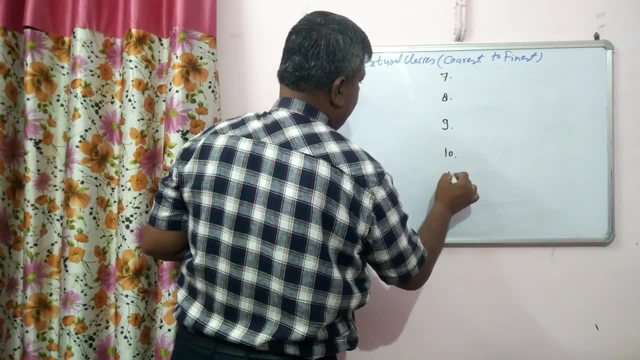 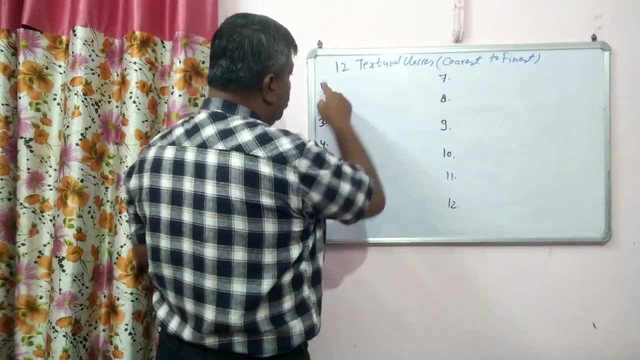 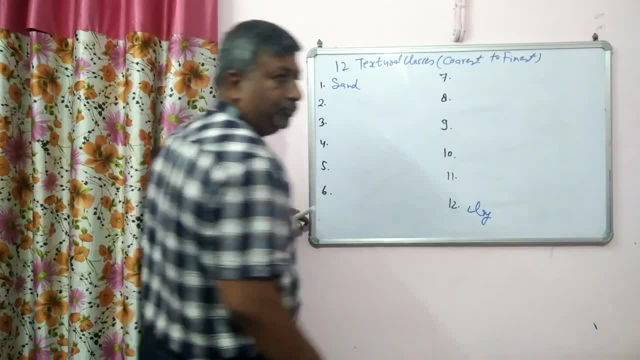 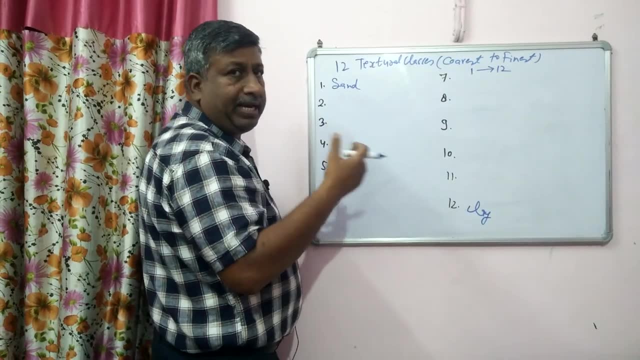 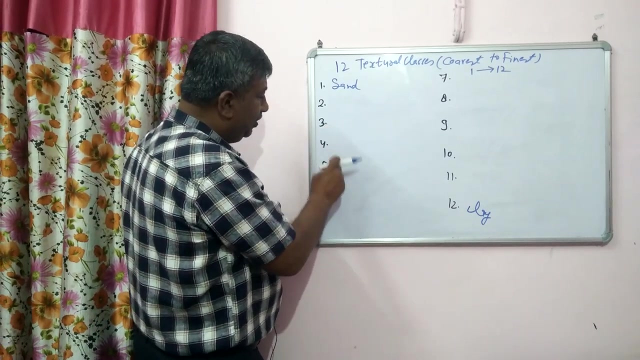 most finest is clay, write here. so this grouping from 1 to 12, which is going on. 1 to 12 means coerceness is decreasing and fineness is increasing. so, as we will see, this is finer, then third one is more finer than 2, then fourth one is more finer than 3, fifth one is more finer. 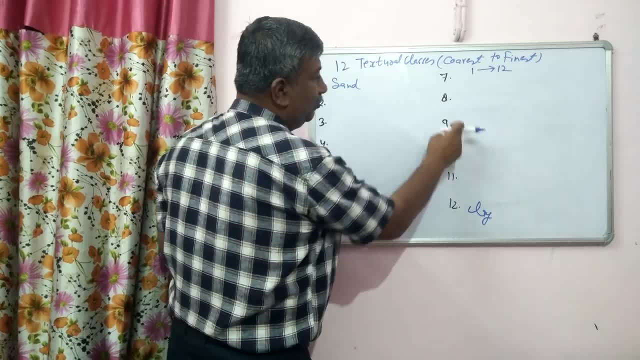 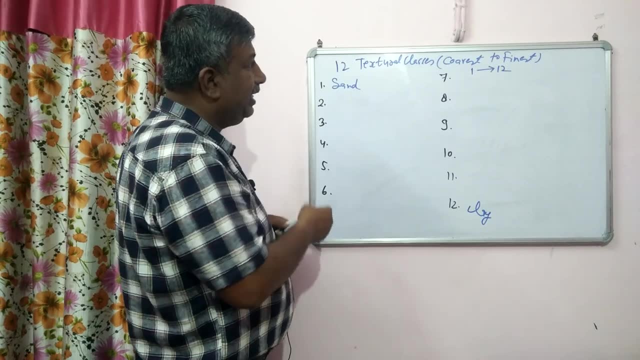 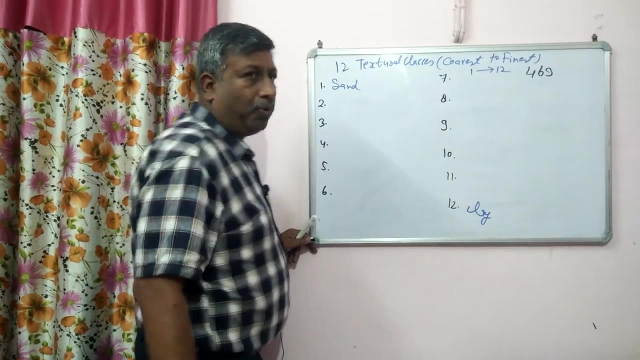 than 4, 7th is more finer than 6, 10th is more finer then 9.. The group of fineness is increasing and texture is getting fine. in this way. we will write then: remember the number 469, 469. just remember the number 469 and mark that number: 4, 6, 9. 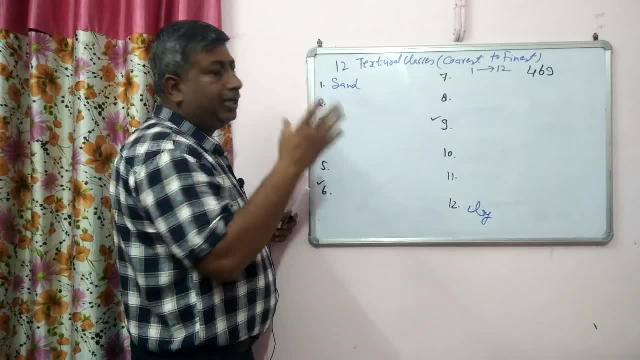 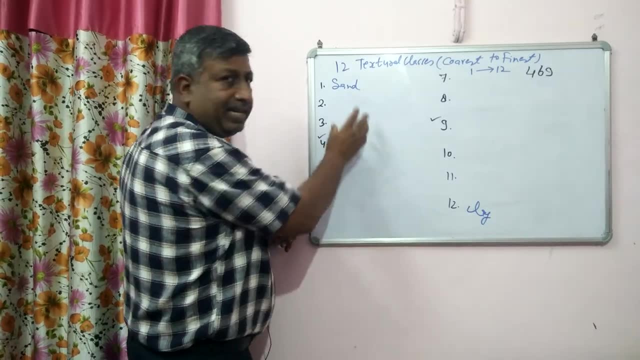 so first I told you that the textual classes are that we will write most coerced, then second coerced, then second coerced, then second coerced. This is the least coarse We can say, that the fineness is increasing, The texture is getting finer, from 1 to 12.. 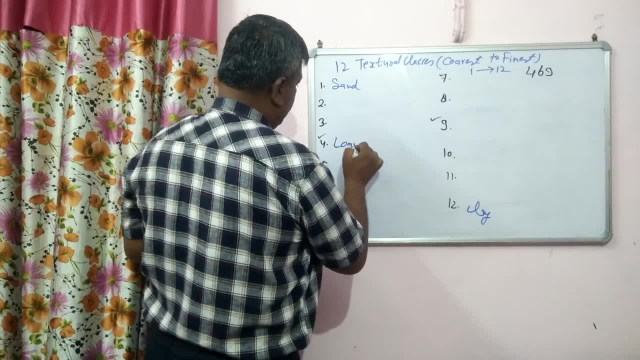 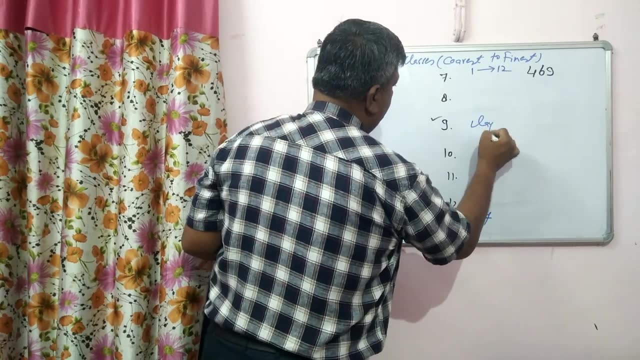 Then here write loam, You have to write loam. here. Here you have to write silt, And here you have to write clay loam, You have to write clay loam. How much work do you have to do? You know sand and clay. 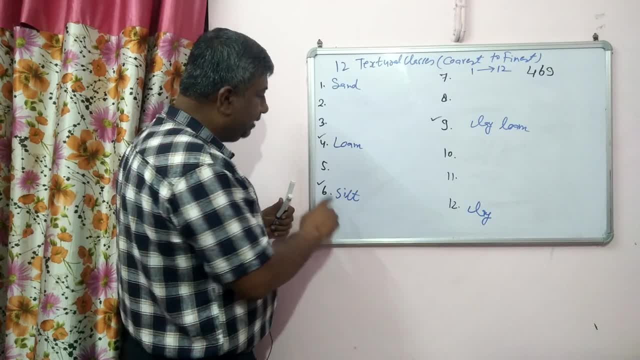 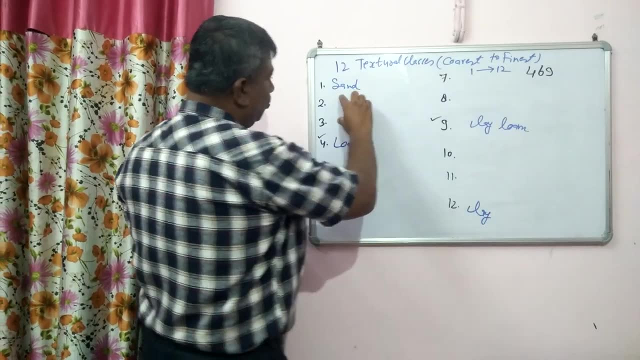 There is sand at the top, Clay at the bottom, Loam at 4.69.. Silt at 5.69.. Clay loam at 5.69.. These group are between sand and loam. Actually write loam above loam. 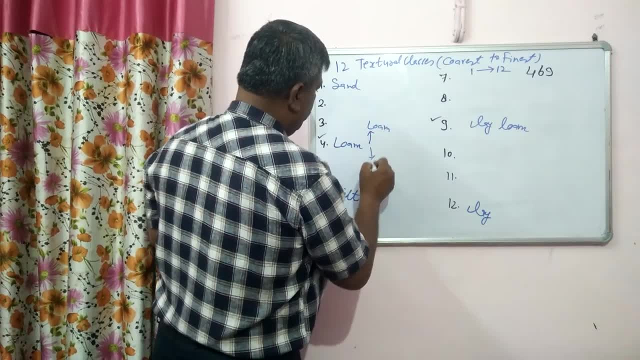 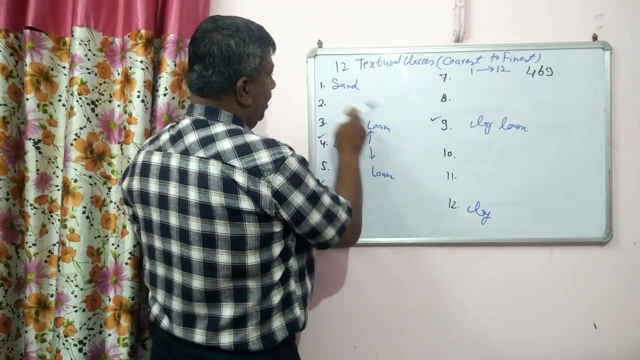 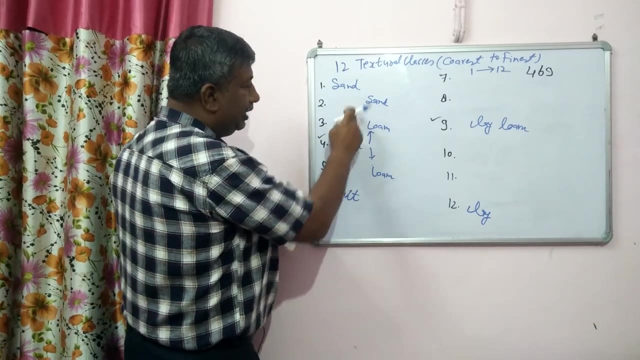 Write loam below loam. You have to do it this way: Write loam above loam and below loam At this soil, Write sand below it, At this intermediate between sand and loam. This is the sand and some part of loam. 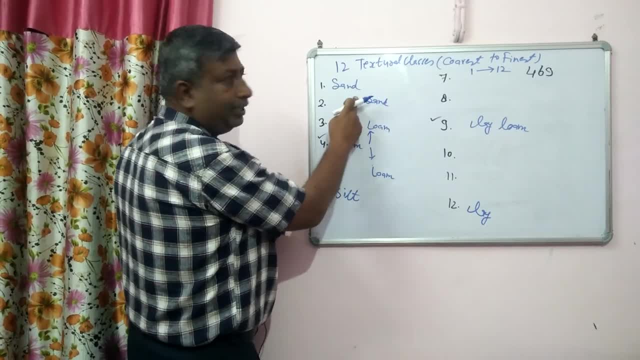 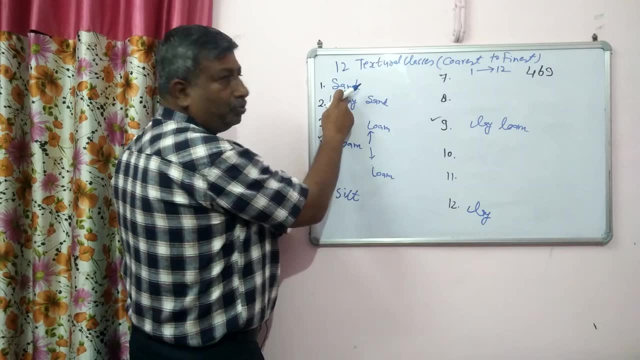 There is sand and loam here, but the major part is near sand. so this is sand and there is some loam in it, so it is loamy sand. second group is close to one, so basically it is sand, but some part of loam is mixed. 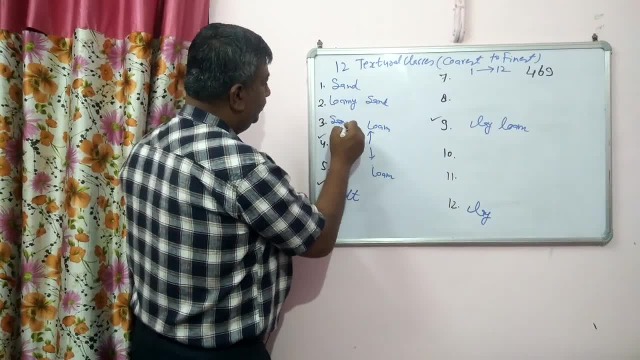 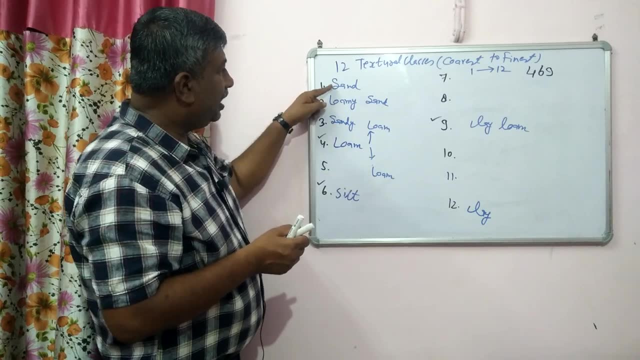 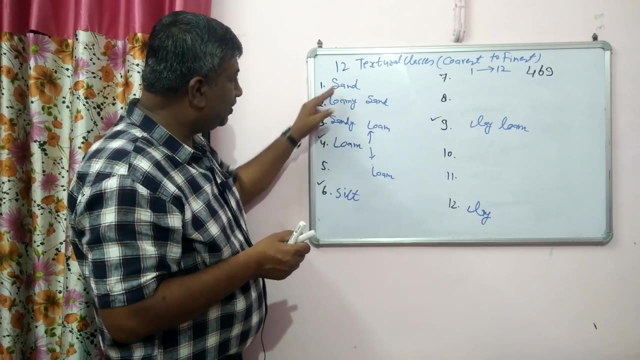 that's why it is loamy sand. here is loam and sand is mixed, so it is sandy loam. this is the easy way. again, i wrote loam loam above loam loam below loam loam above loam loam below loam. 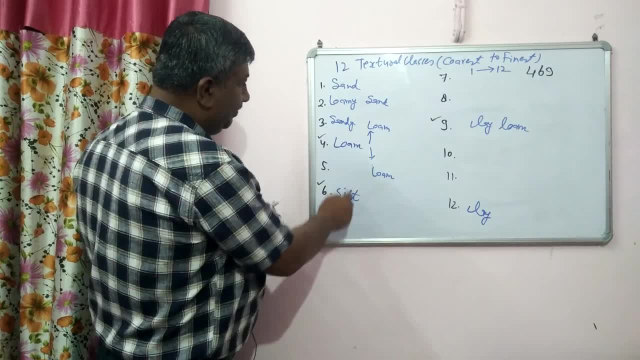 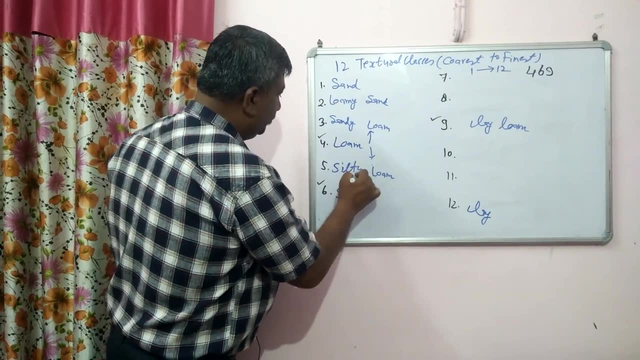 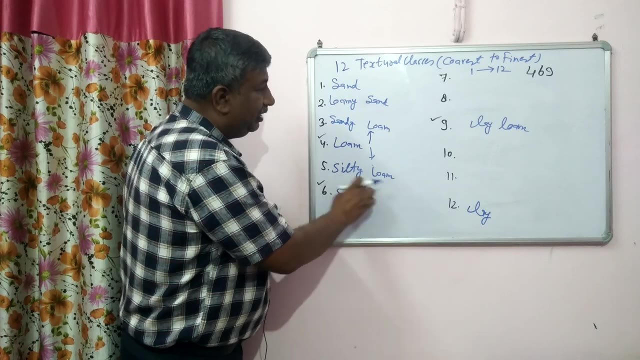 sandy loam and this is the between silt and loam. i wrote: loam and silt is mixed. silt is silt loam. this is loam. silt is silt loam. it is silt loam. some part of silt. 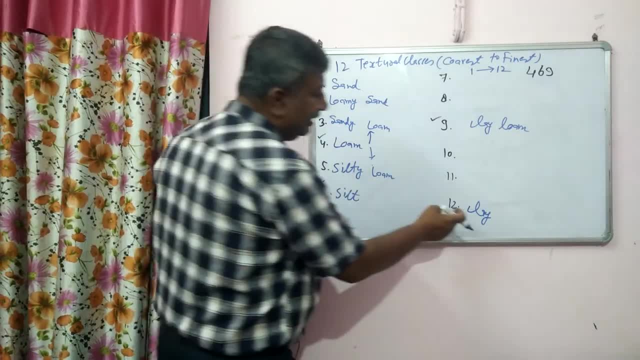 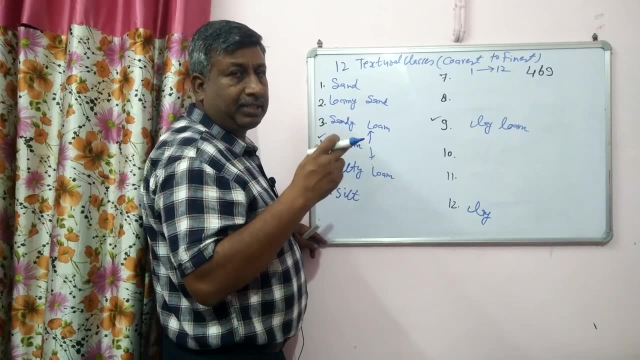 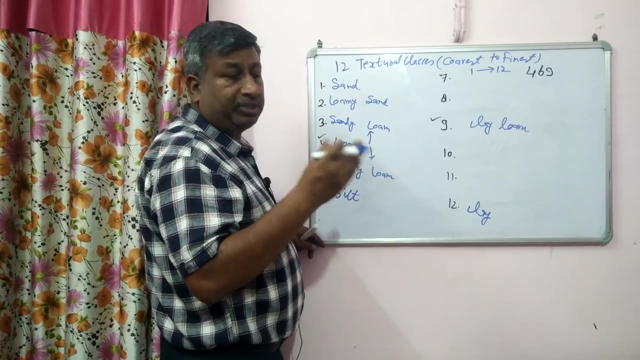 so that's why it is silt loam. we have written it like this. we will start from the bottom. clay is fine, sand silt and clay most coarse is sand, then finer is silt and most finest is clay. if i say clay is coarser, then it is silt. 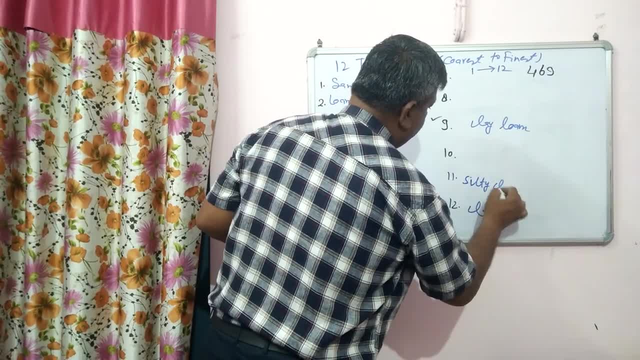 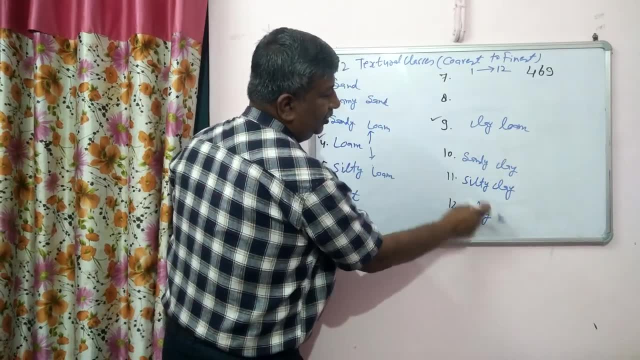 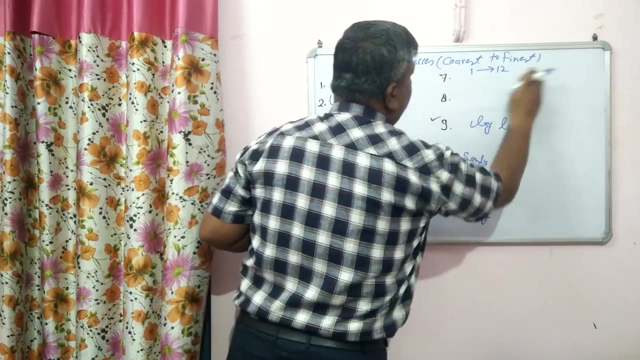 so silty clay coarser than that sandy clay. sandy clay. here we started from clay, here we have to coarser, because here coarseness is increasing opposite. see, coarseness is increasing from 12 to 1, so we will go from 1 to 12. 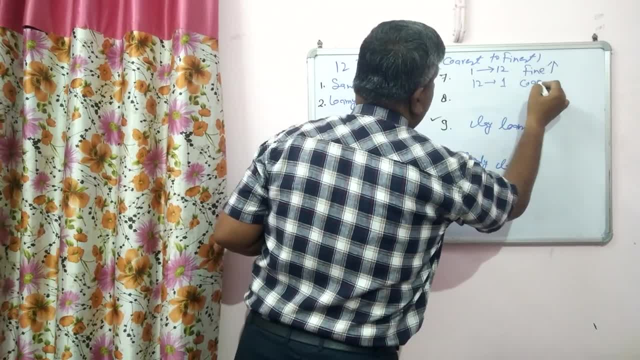 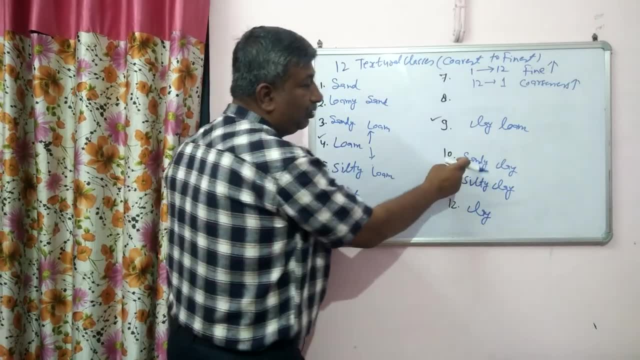 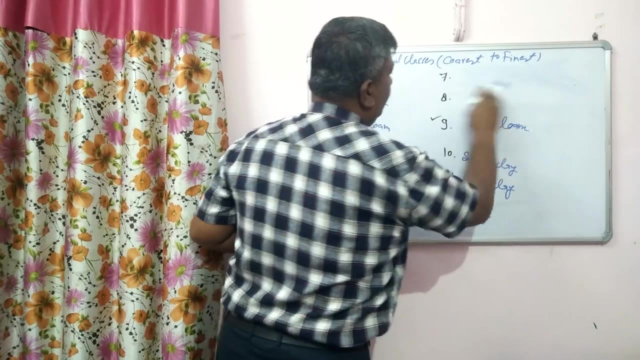 and if we go 12 to 1, so coarseness will increase. coarseness is increasing, so coarseness will increase. so first we will add silt, then coarseness will increase here. clay is loam, so see if i want to coarser clay loam. 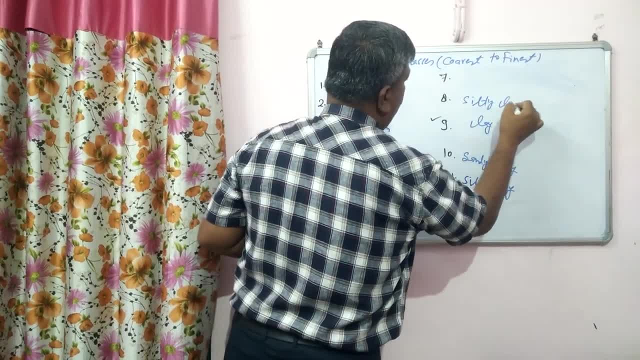 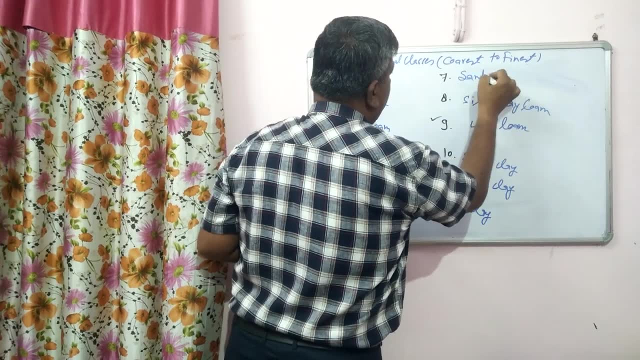 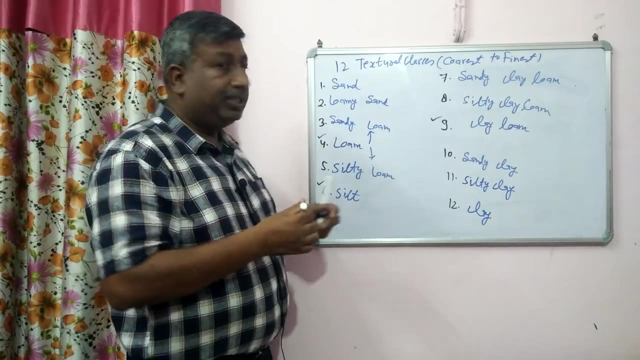 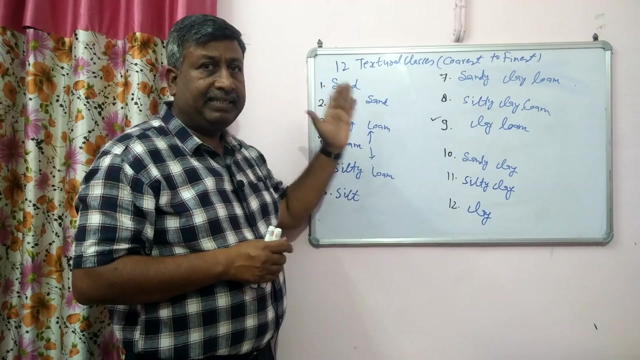 then what will i add? first, i will add silt. i wrote silty. now i have to coarser it more coarser, so it is sandy clay loam. so this is the way how we can write that different 12 texture classes according to their coarseness and fineness. so 1 to 12. fineness is increasing and 12 to 1. 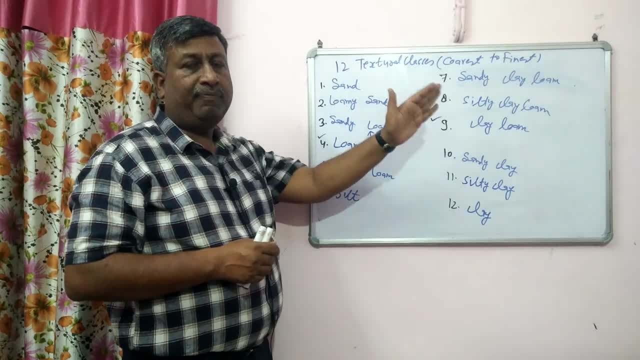 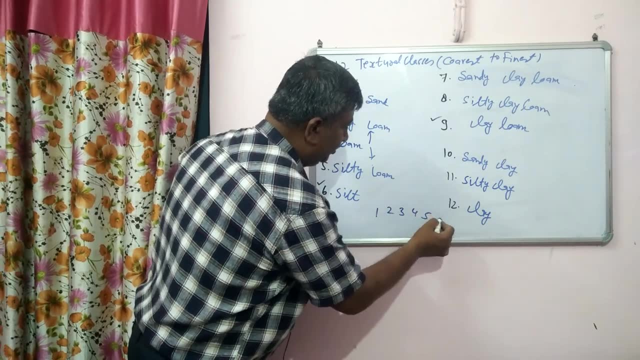 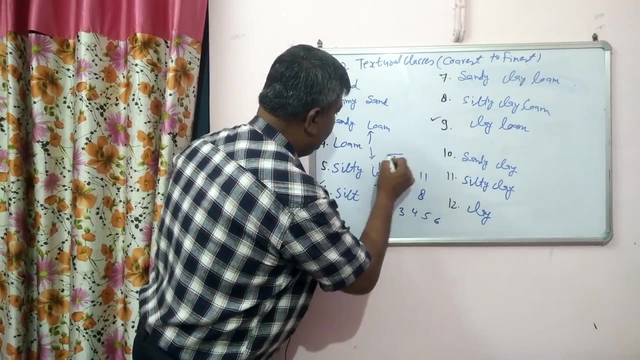 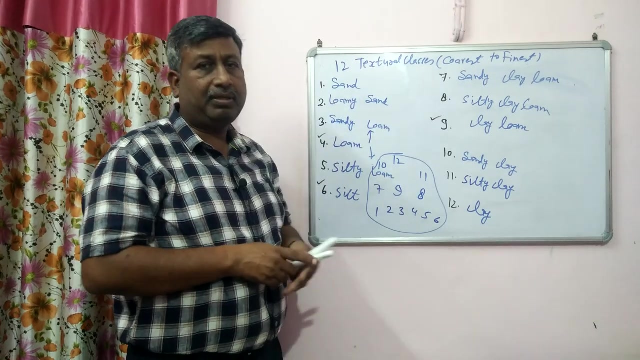 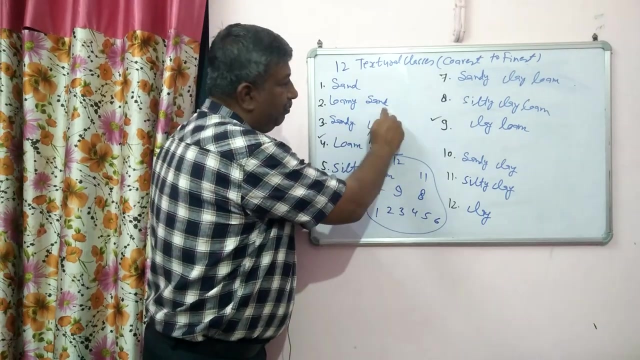 coarseness is increasing. so according to this texture classes, you can find out which one is more coarser. so we have to find out if loamy sand is more coarser or sandy loam. so we will find out from behind, back, back, see the back. 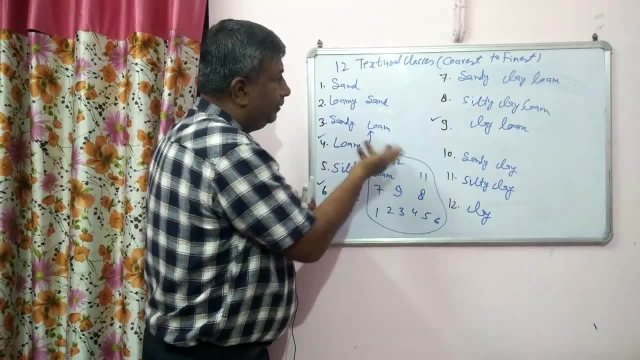 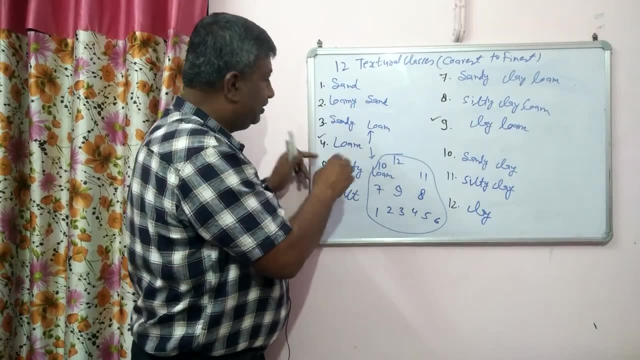 which one is more coarser: loamy sand or sandy loam. it may be confusion, so compare last word. so sand is coarse, so it means loamy sand is more coarser than sandy loam. similarly, we have to find out if we want to compare silty loam and silty clay loam.